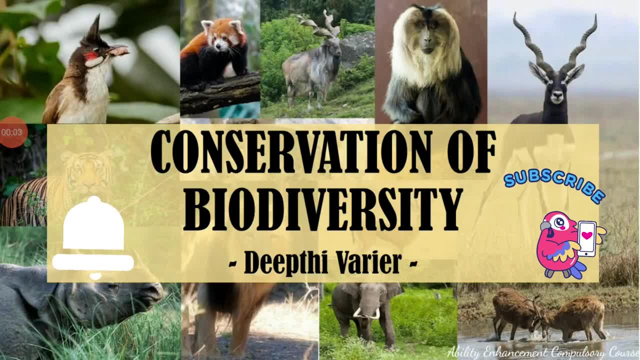 Hello and welcome to my channel. As we know, biodiversity refers to the diversity or variability among living organisms in an ecosystem. But this biodiversity is under threat due to various human activities. So the concept of conservation of biodiversity was stressed upon in the Convention on Biodiversity in 1992, so that a sustainable development can come about. 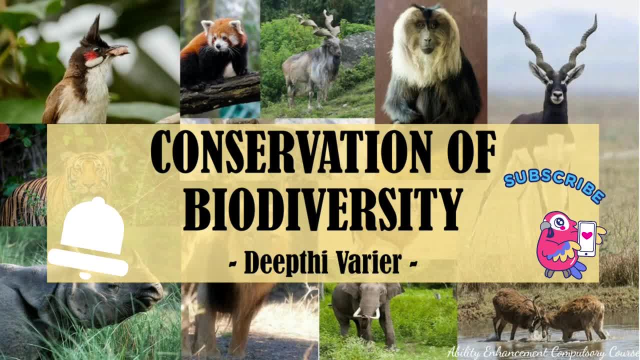 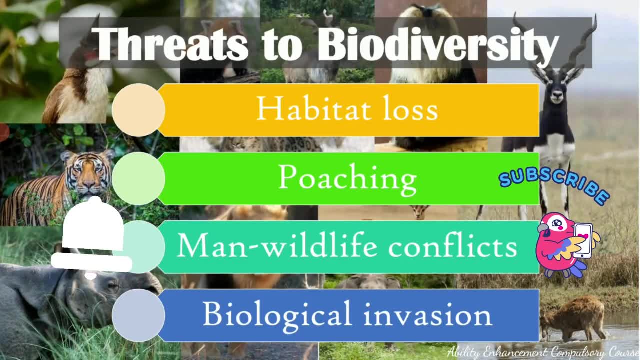 and there is perpetuation of human beings on earth. In this video, we look at what is actually threatening biodiversity and what are the different conservation strategies that we can employ. Now, the main threat to biodiversity comes from the loss of habitat, The reason being we. 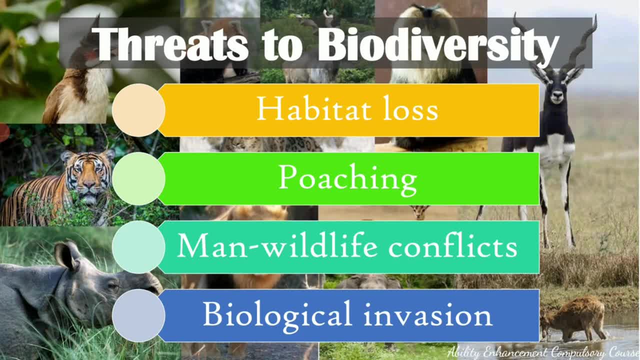 humans use up the habitats or use up the forest land for various purposes, like the agriculture, or for industrialization, or for building settlements, for urbanization or in some cases there is fragmentation of the habitat, So there is loss of the habitat in installments and it. 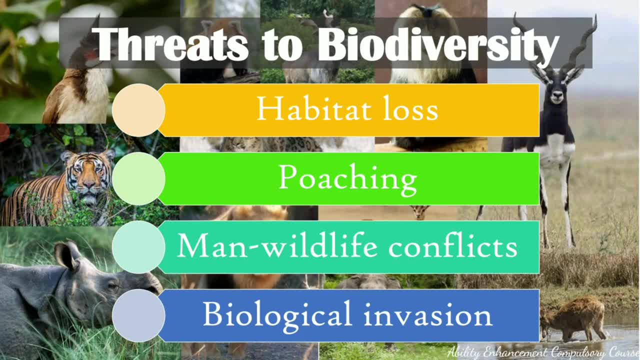 leads to scattered patches of the forest or scattered patches of the habitat, which all together is a huge threat for the biodiversity. Not only that: certain area, certain ecosystems, like marine habitats or even the wetlands, are subjected to very high pollution. So there is some kind of human intervention which is upsetting that habitat or due to which the 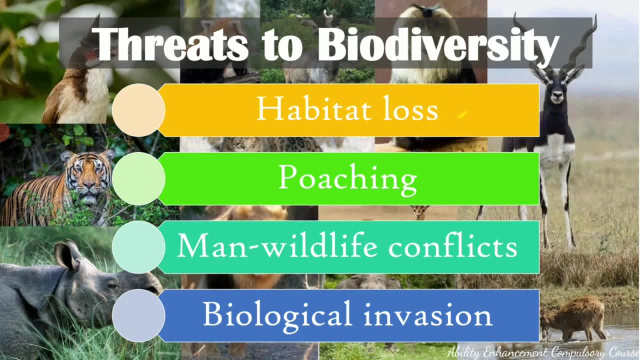 original habitat is getting lost, and that is a big problem, due to which the biodiversity is also getting depleted. The second reason for the biodiversity to be under threat is poaching. Poaching, the hunting, the harvesting of wild plants and animals, illegal trade in their 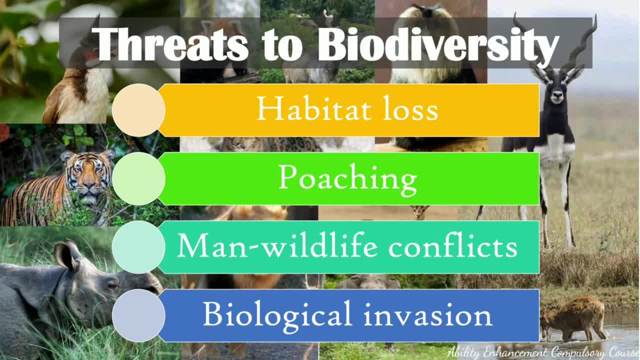 products, like for the horns or tusk or fur or their meat. In some cases, certain plants- exotic plants are, you know, cut down for making up herbal products. So all of these reasons, the illegal hunting down or cutting down of plants and animals is also leading to their loss, or is. 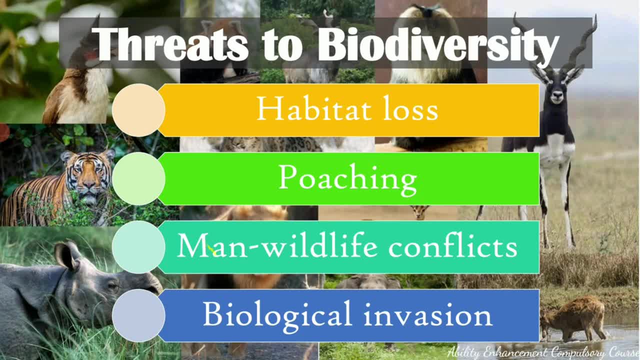 also acting as a threat to biodiversity. The third reason is man- wildlife conflict. Man and wildlife have been, you know, hitting against each other. They have been in conflict due to many, many limitations on the resources. There is limitation on the food. There is. 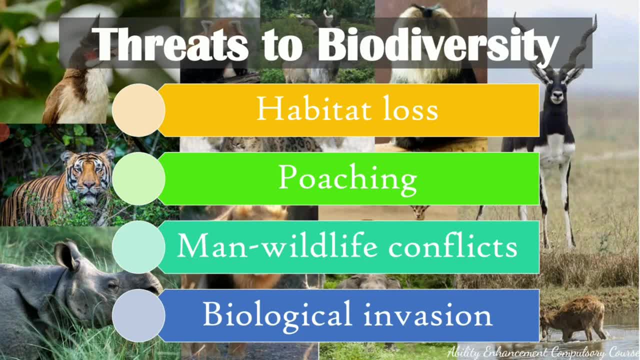 limitation on the water resources, There is limitation on the habitat. So, due to all of these reasons, the wildlife and man has been in a perpetual conflict and that is a big reason for loss of biodiversity, The reason being when wildlife enters into the human settlements. 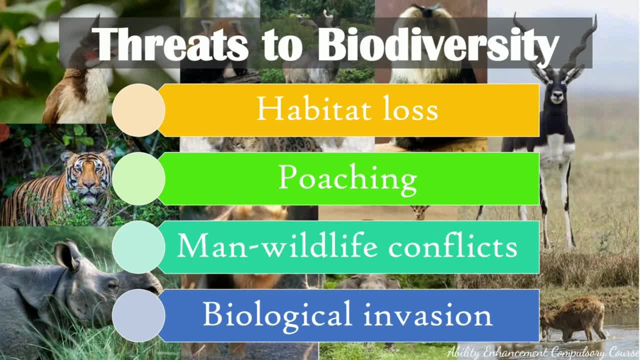 humans get back into the wild, They get back into the wild, They get back into the wild, They get back, and there is a lot of revenge, killing that happens, or they even trap the animals, So that leads to the animals getting moved out from their original habitat or from their natural habitat. 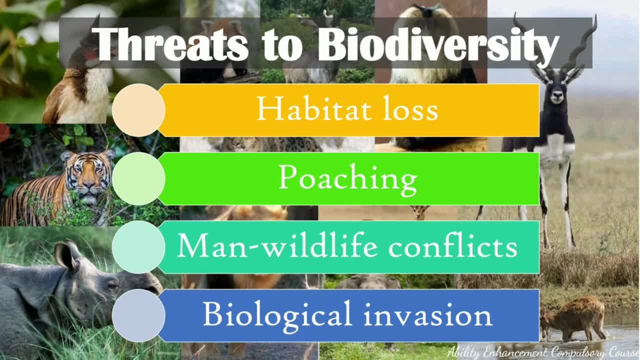 The last reason for the threat to biodiversity is biological invasion. Now this includes the rapid expansion of a species into a region where it had not previously existed. That is, it has been introduced accidentally into a particular region, but in that region it has taken over the native flora and is now spreading far and wide. A very good example for 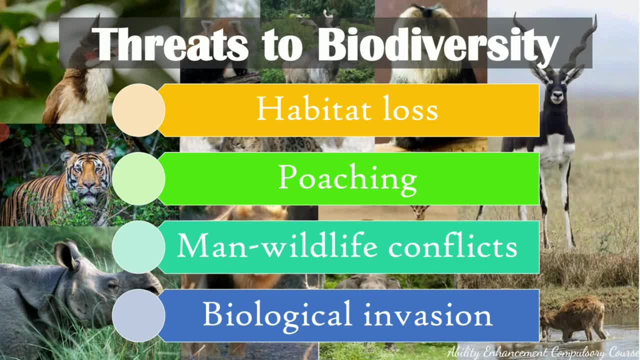 this is the wheat Parthenium which was introduced into India from US in the 1950s through wheat plant. So it was a contamination through the wheat seeds and that is how we got Parthenium in India. but now Parthenium is present everywhere. It is acting as a complete weed and growing. 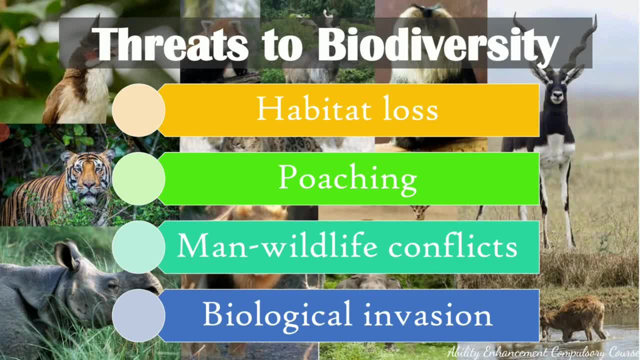 in all parts of the Indian subcontinent. So these are the four major reasons for threat to biodiversity: The loss of their habitat, illegal and rampant poaching man, wildlife conflicts that keep occurring and biological invasion by other species. Now, due to this, there has been a lot of pressure on biodiversity in many parts of the world. The number of endangered 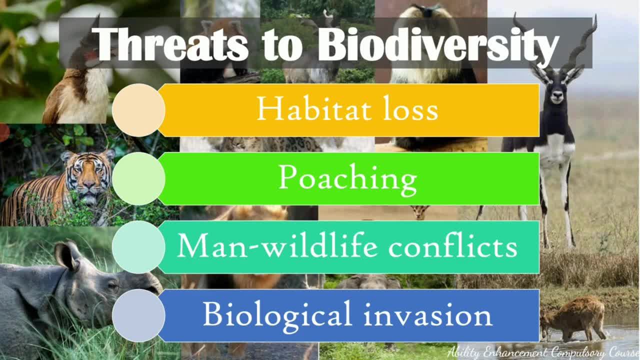 species has gone up, A lot of species, have you know. some of the species have become extinct, or at least extinct from the wild. So, to make sure that this doesn't go on further, to make sure that we are able to, you know, conserve our biodiversity, The conservation of biodiversity has been taken. 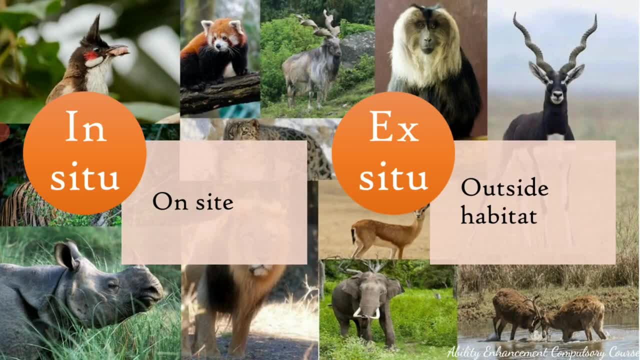 up very seriously by government and by the government. So this is a very important point. Now there are majorly two categories or two types of conservation strategies. We can have on-site conservation strategy, that is, conservation of the ecosystem, conservation of the natural habitat, maintaining and recovering the viable population in their natural surroundings. 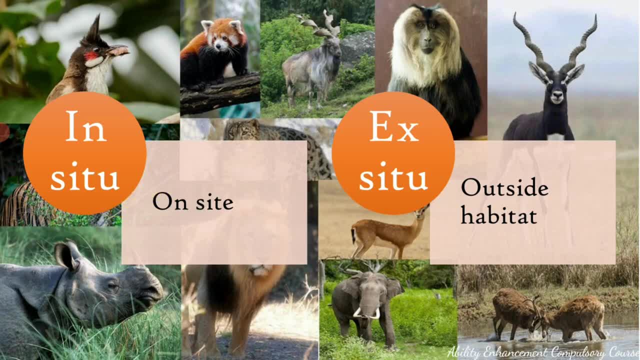 That is called as in-situ conservation strategy. The other type of conservation strategy is ex-situ, which happens outside the habitat. So you conserve the components of the biodiversity, but away from their natural surrounding, away from their natural habitat. So let us look. 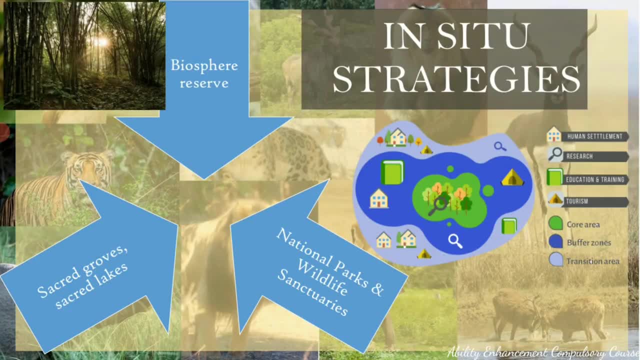 at each one of these in detail. In-situ strategies includes examples like biosphere reserve. Now, these biosphere reserves are large areas which can have other national parks or wildlife sanctuaries inside it, So these are basically undisturbed areas which are used for research. 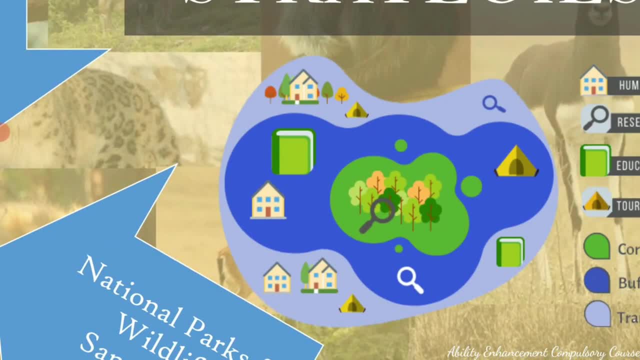 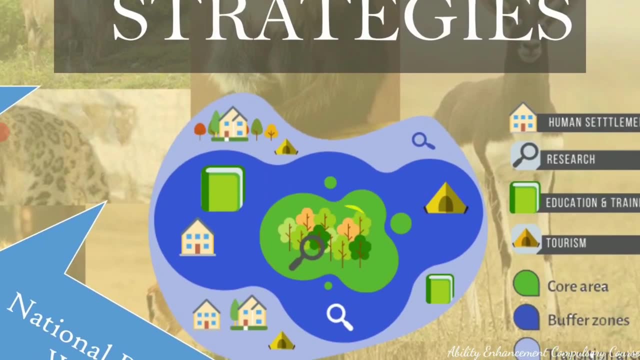 and where you have the biodiversity thriving very well. This, what is shown over here, is how a biosphere reserve looks like. So you can see here that the innermost region of the biosphere reserve is the core zone. That core zone is the zone which lacks human activity, So it is exclusively 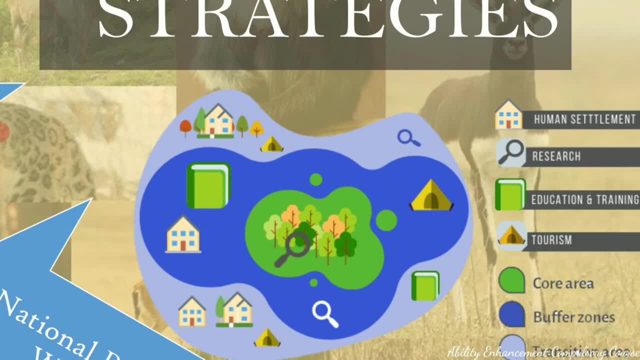 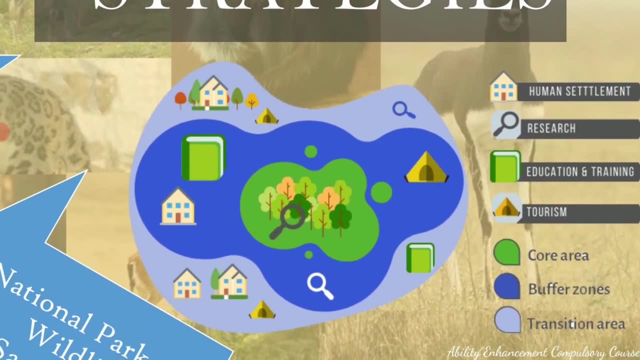 for the animals and the plants, for their preservation, for their conservation. The core zone is surrounded by a buffer zone, the one which has been shown in dark blue here. Buffer zone is the zone where there is a bit of ecotourism, a bit of grazing is allowed and research is also. 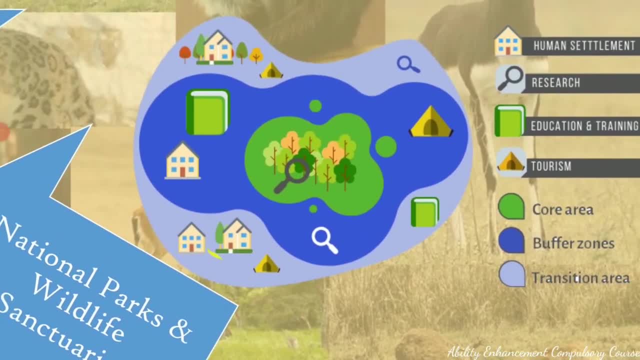 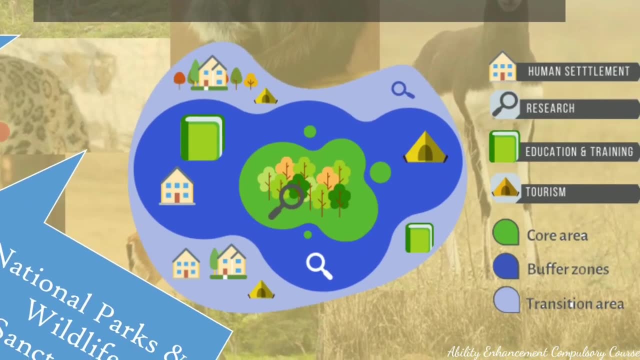 allowed. The last zone of a biosphere reserve, the area which is the outermost area of the biosphere reserve, is the transition zone. It acts as a transition between the biosphere reserve wildlife and the other settlements that are there in that region. That's why. 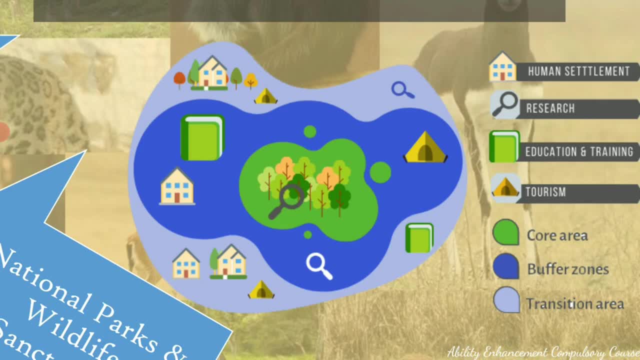 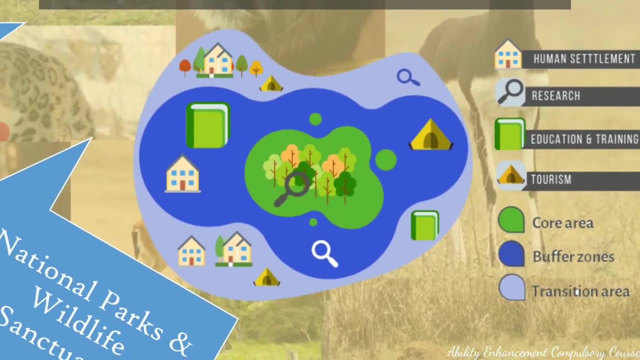 it's called as a transition zone. So it allows human settlements, it allows crop cultivation, it allows grazing and, of course, research and tourism. So this is the transition zone. We have the buffer zone and we have the core zone. This is how a biosphere reserve looks. 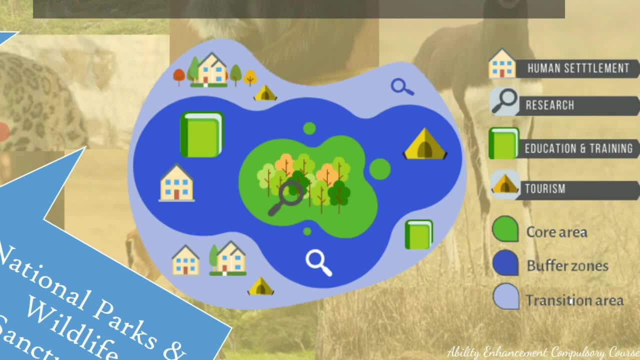 like Now. having a biosphere reserve is a very good thing, because it not only helps us to preserve the habitat, it helps us to preserve the flora, the fauna and also the communities which are attached to that particular region, So it helps us to sustain their ways. 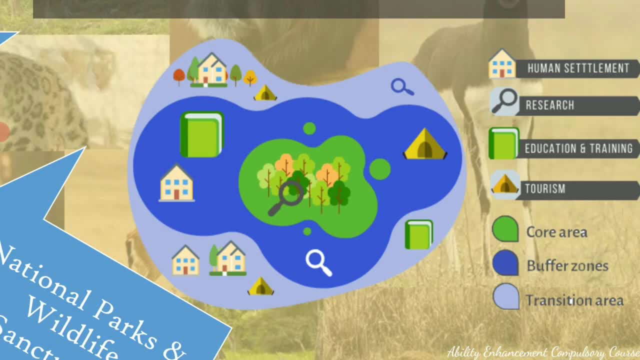 of life. Their livelihood is preserved by a biosphere reserve. In fact, biosphere reserves were included under the Biosphere Reserve Network Program by UNESCO, which in 1971 it was launched by UNESCO under the Man and Biosphere Reserve Program And under that India is having. 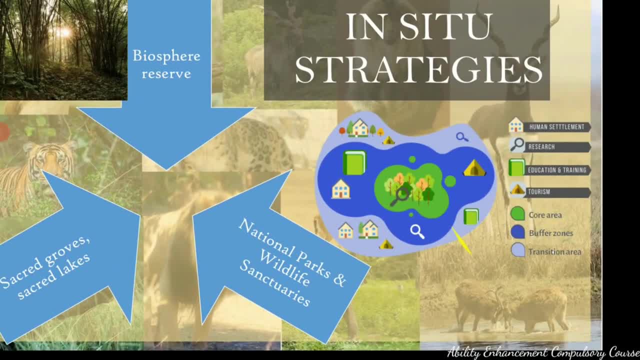 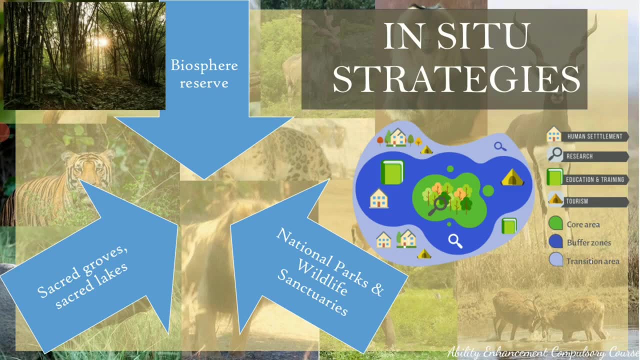 as of 2022, India has 18 biosphere reserves, So these biosphere reserves are a very good in-situ strategy for protecting the biosphere. So this is a very good strategy for protecting not only the flora and fauna, but also the ecosystem, the environment. Nilgiris was. 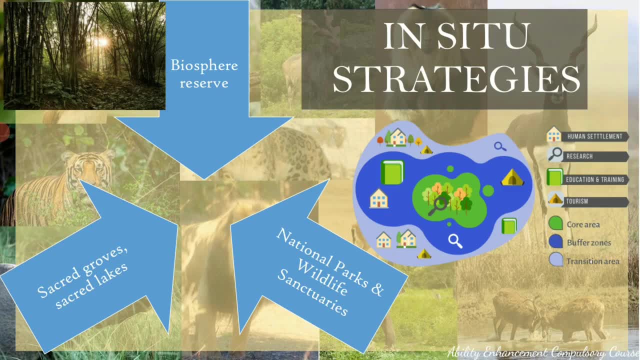 the first biosphere reserve in India. We have many, many others as well. The second type of conservation for or under in-situ conservation strategy is having national parks and wildlife sanctuaries. So as of 2022, national parks are 106 in number in India and we have more. than 565 wildlife sanctuaries, So we have a huge number of wildlife sanctuaries and national parks. The difference between these two terms is that national parks aim at protecting the ecosystem, So they are much larger, whereas wildlife sanctuaries are aimed for protection. 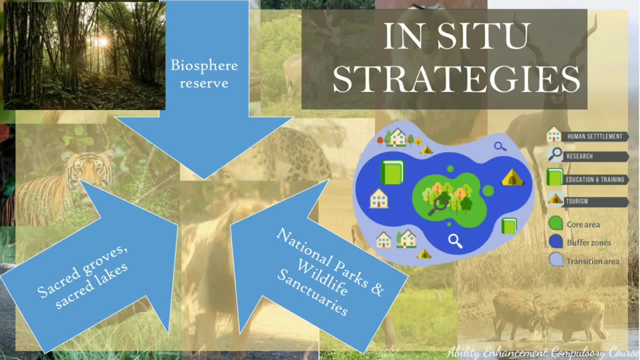 of the animals, So they are slightly smaller, but both of them are equally serving the purpose of conservation. One of the examples of national parks that we have around the state or in the state of Karnataka is the Banerjee Ghat National Park, which is in Bangalore, or we. have Bandipur National Park, Nagarhole, Kudremukh, And we have a lot of national parks in the state of Kudremukh And one of the wildlife sanctuaries that we have very close to the city of Bangalore is the Ranganthitu Bird Sanctuary. So these are the second type of conservation. 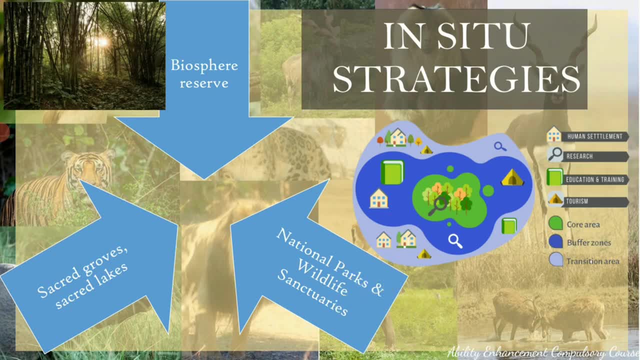 strategy that is having national parks and wildlife sanctuaries. The last type of in-situ conservation strategy is having sacred groves and sacred lakes. Now, these are areas where they are like a protected refuge that are present. It's not only in India, we even have 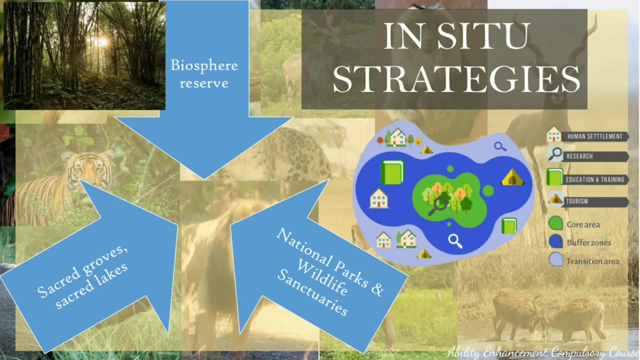 it in other countries, like in Ethiopia. They provide shelter to many rare species of flora and fauna. They act as water sources for the local villages. So these growls or these patches of forest are considered to be abodes of deities by the local communities, by the rural communities. 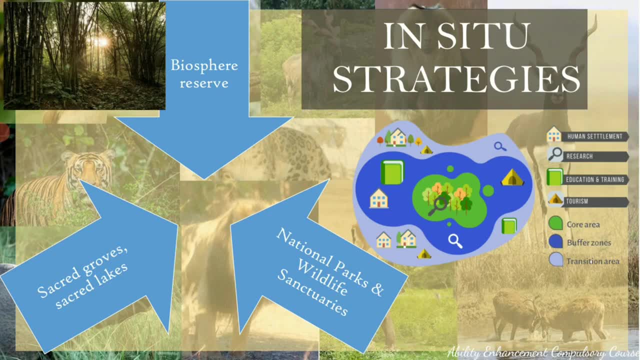 And that is the reason these people protect that particular region in a very Holy, because they are considering it Holy. that region and its ecosystem is well protected. Some examples of this include the Khasi hills of Meghalaya We have. the one shown here is the Ponad Kadia. 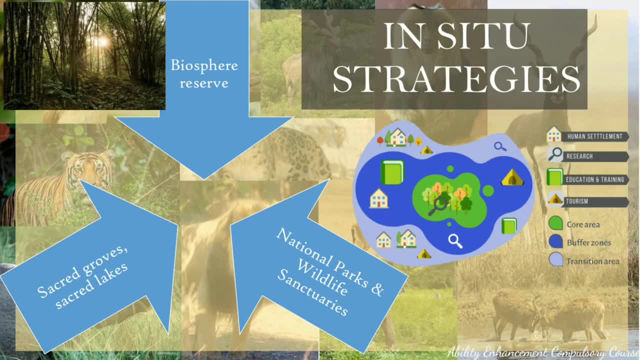 It's a sacred grove. In Maharashtra we have the Aravalli hills of Rajasthan. They're all considered sacred and due to which they're all conserved like that They're not. you know, there is not much of human habitation in such areas. 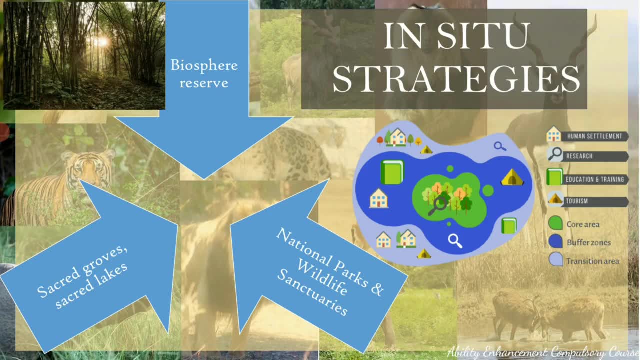 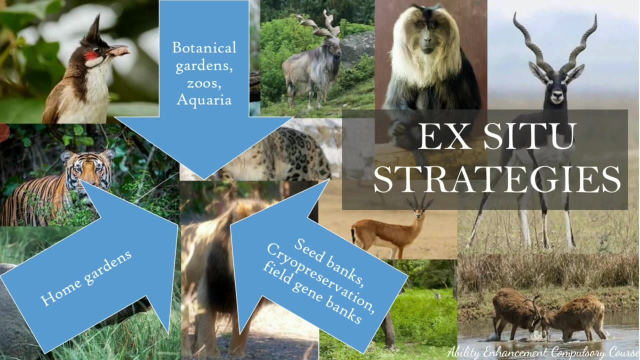 Even in Ethiopia we have a lot of forests where there are churches inside the grove, So that makes it holy and it is protected by the local people. These are the in-situ strategies, or on-site strategies. When we look at ex-situ strategies, it includes the strategies for protection of the biodiversity away from its habitat.